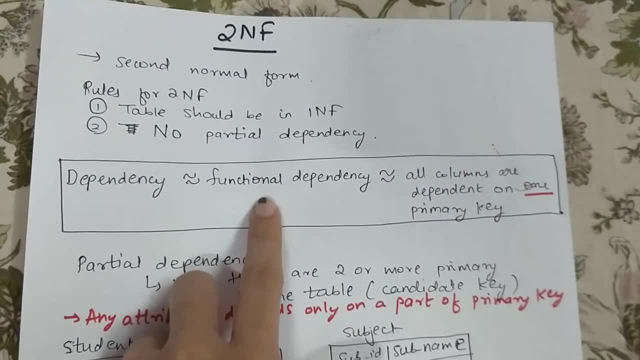 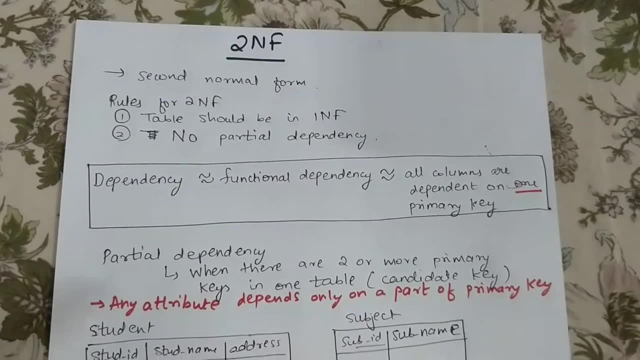 is also known as functional dependency. It is same as functional dependency and what it basically means is that all columns in a table are dependent on one primary key. Now, for example, if you see this table- student table- there is a student id, student name. 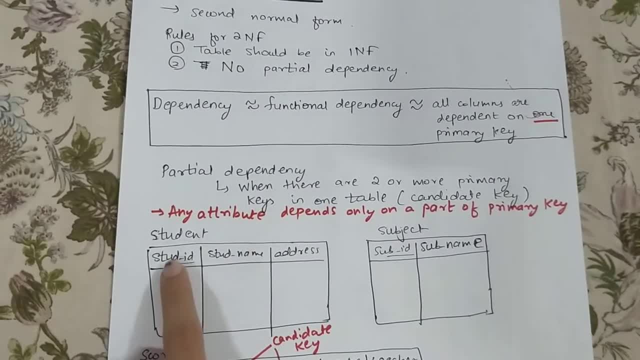 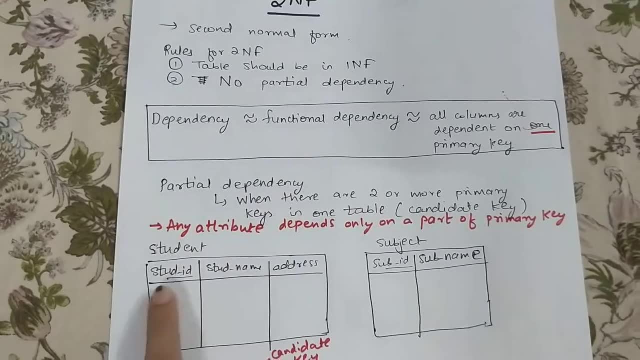 address, Now student name. the primary key is student id, Now student name and address. both will depend on student id. Basically, all the other columns are dependent on one column, On one primary key, And this is what functional dependency is, Now partial dependency is. 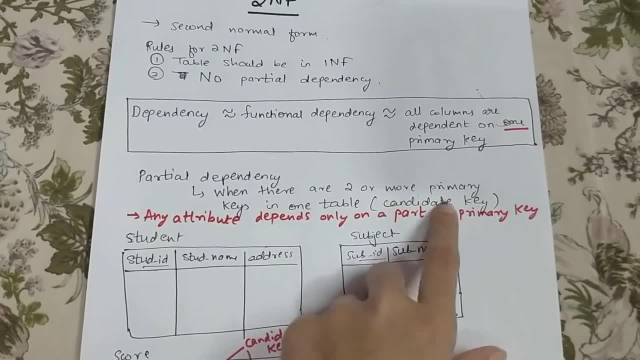 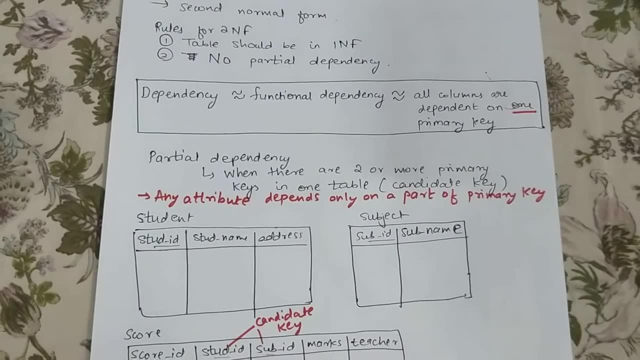 what is it Now? partial dependency happens when there are two or more primary keys in one table, Basically when there is a candidate key. We have already discussed what candidate key is. Any attribute depends only on a part of primary key, Okay, and not on the complete. 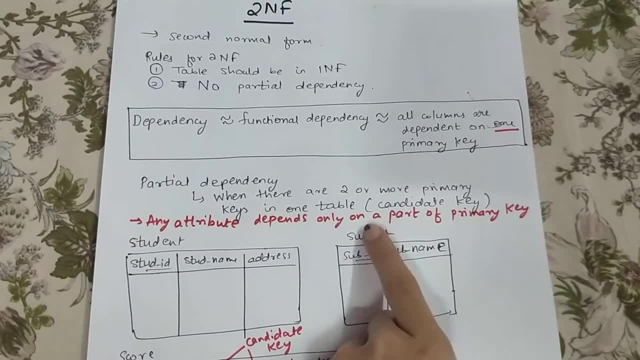 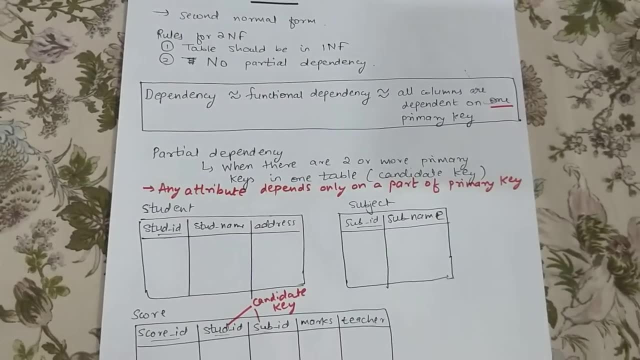 primary key. Basically, it depends only on a part of a candidate key and not on the entire candidate key. Okay, This is a mistake. This should be candidate key. Okay. So what this means is I'll explain. So there are three tables: Student table. subject table: 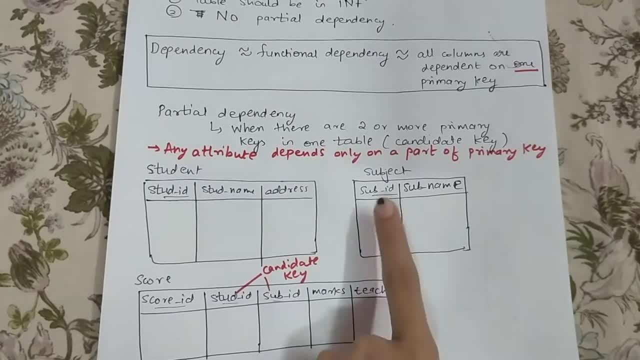 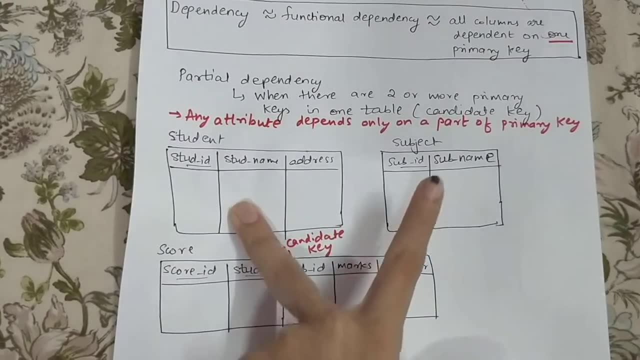 score table. Now student table has student details and subject table has subject details, subject id and subject name. Now there is a score table which has score id, student id and subject id, which are linked to these two tables. Okay, And then there is a marks. 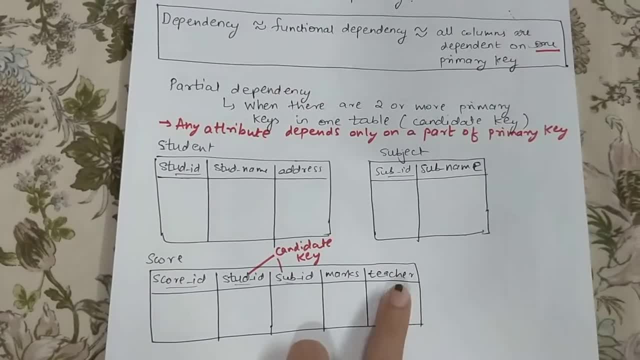 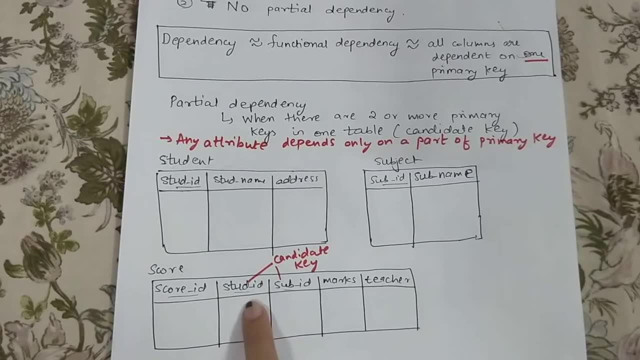 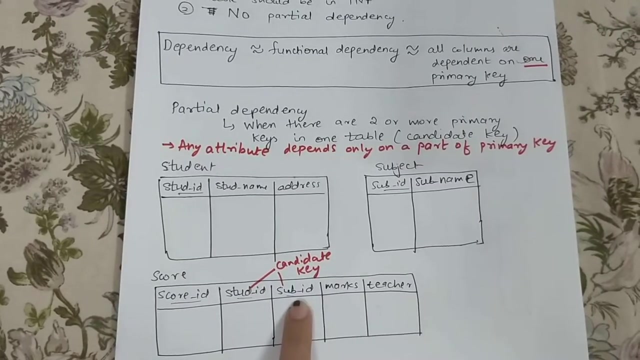 column and there is a teacher column. Okay, Teacher column is basically teacher's name And marks. So in this table there are two primary- this is the basic primary key- and these are also candidate keys- Student id and subject id. So basically there are three. 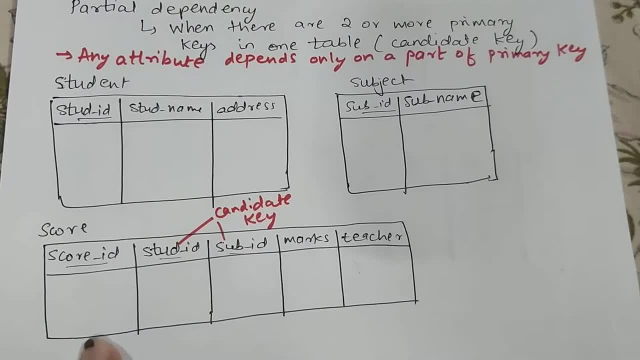 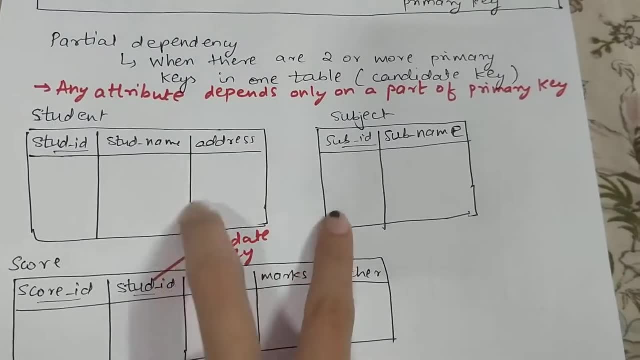 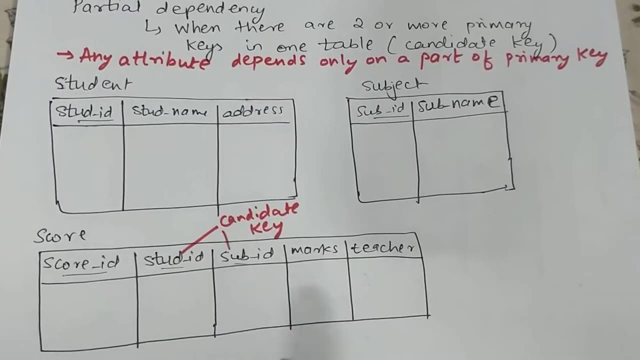 primary keys in this table. Okay, Now, score id will uniquely identify each row in this table, and student id and subject id are the keys which will link to these two tables. Okay, Now, marks are marks and teacher name. Now, if we see these, these are primary keys. Now, marks. Marks is a non-prime key. Now what? 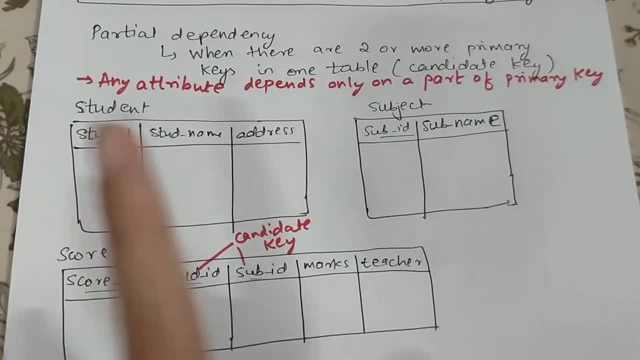 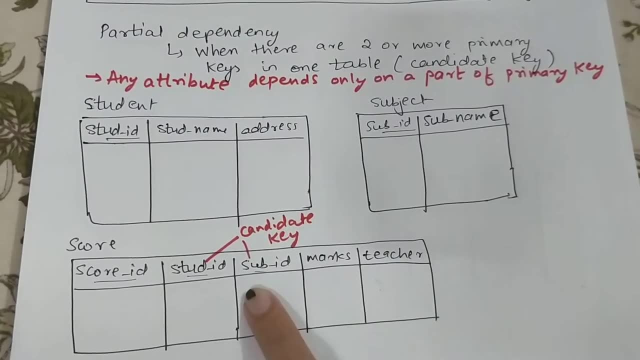 are prime keys and non-prime key. No, Prime keys are the primary keys and non-prime are the. basically all the other keys except the primary keys, Okay, So marks: marks is dependent on subject id: Yes, Marks is dependent on student id: Yes, So there is dependence. No.